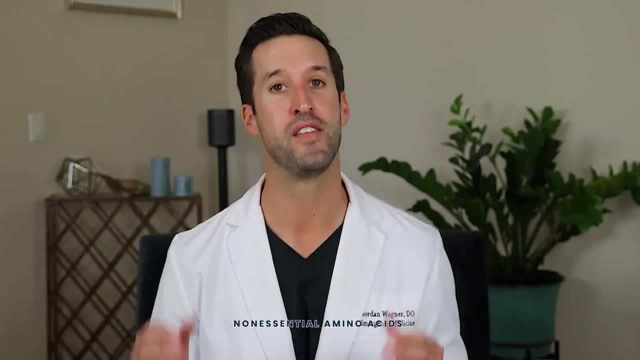 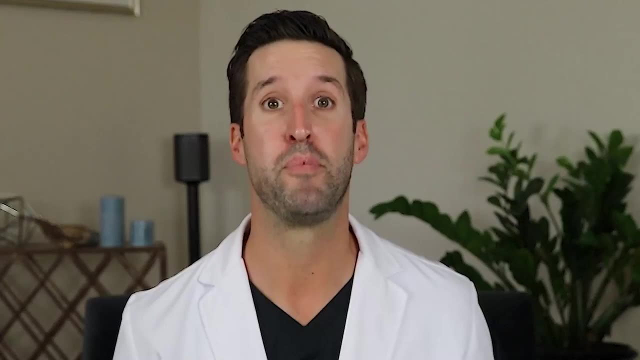 classified into three groups: essential amino acids, non-essential amino acids and conditional amino acids. What we're really going to focus on are essential amino acids. Why? Because our bodies can't produce them. like non-essential amino acids, We can only get essential amino acids from outside. 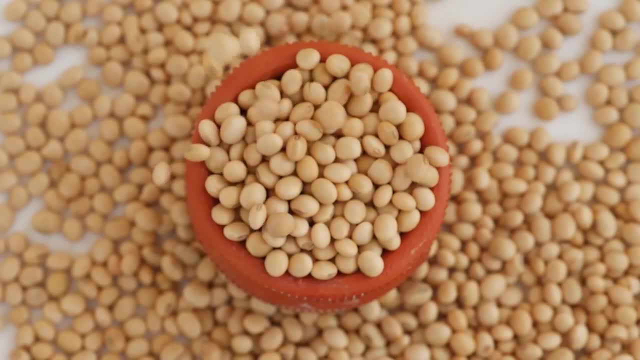 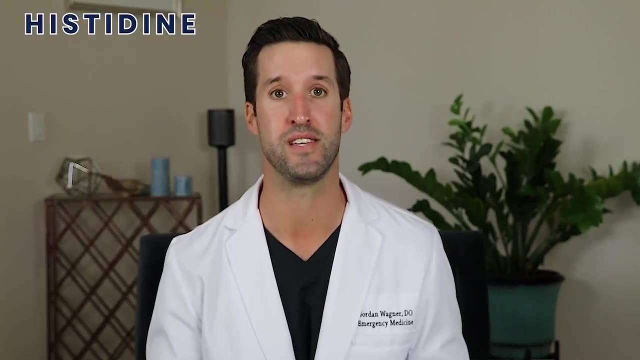 sources such as foods like meat, eggs, quinoa and soy, or a diet supplement drink mix. To break it down even further, there are nine essential amino acids. These include histidine, isoleucine, leucine, lysine, methionine, phenylalanine, threonine, tryptophan and valine. 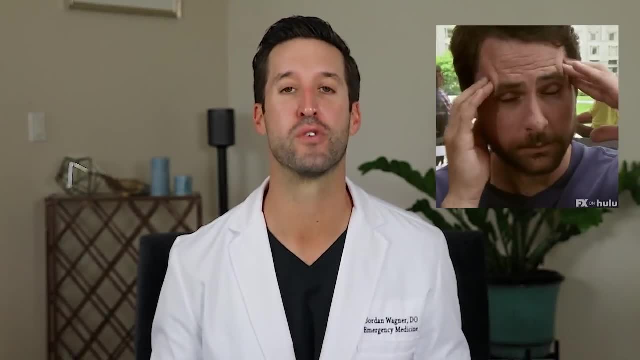 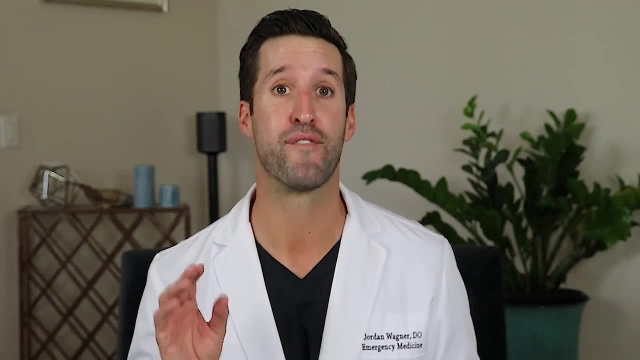 Wow, That's a lot of words. You don't need to know all of those. Just know that they are essential and they are key players in our body's function, as I mentioned before. But what if I told you there are five additional benefits that you probably didn't even know about? Ready to hear? 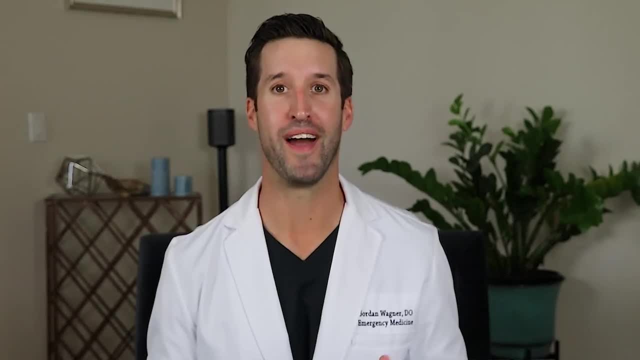 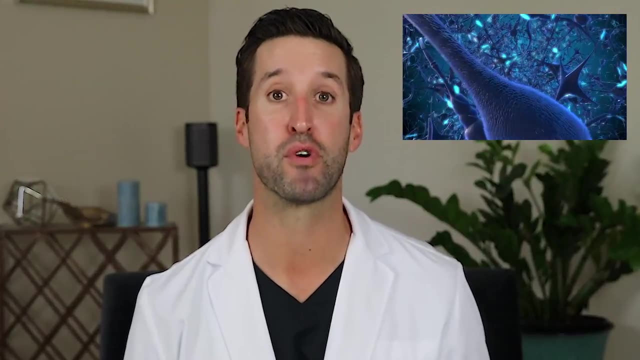 five life-changing benefits of amino acids. Number one: mood and sleep. Tryptophan, one of the essential amino acids, is needed for the production of serotonin, a chemical that acts as a neurotransmitter in your body. Serotonin regulates our mental health. 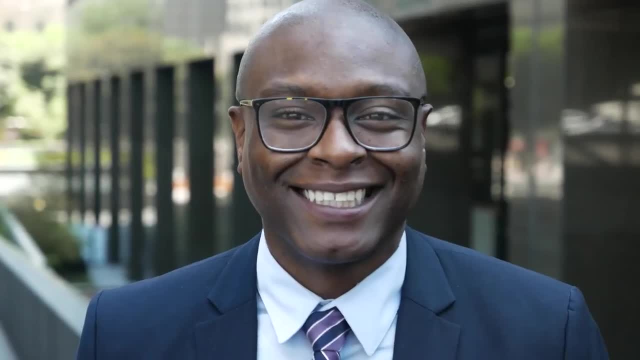 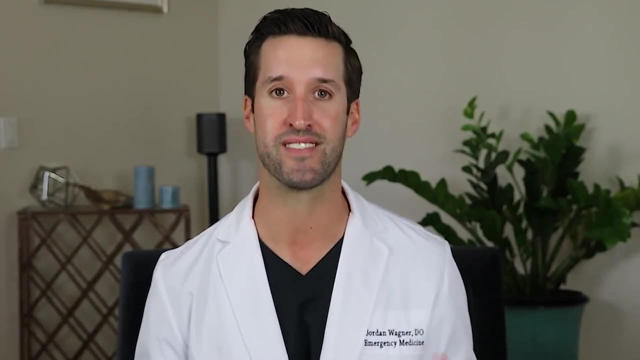 such as our mood, sleep and other day-to-day behaviors When it comes to happiness and how you feel every day. serotonin is also important for reducing depression and regulating anxiety. Several studies have shown that supplementing with tryptophan can reduce symptoms of depression. boost mood and improve sleep. Number two benefit of amino acids you may not know about: they promote weight loss. Yep, Some human and animal studies have demonstrated that essential amino acids may be effective in stimulating fat loss. They are also important for reducing weight. 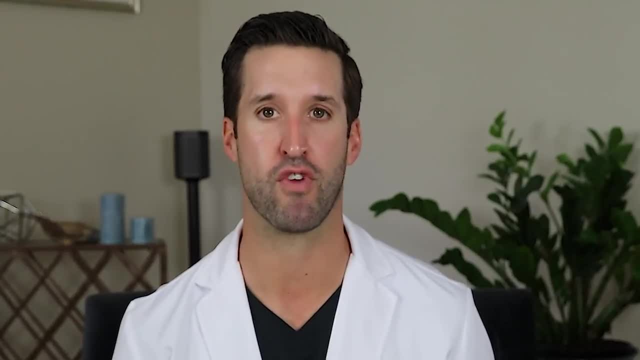 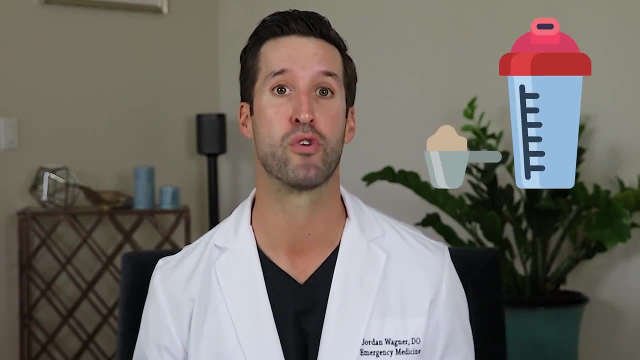 An eight-week study found that supplementing with 14 grams of branched-chain amino acids per day significantly decreased the body fat percentage compared to whey protein or sports drinks. Number three: decreased muscle soreness. It's not uncommon to feel sore a day or two after a. workout. especially if your exercise routine is new, Here's a suggestion: Try sipping on some amino acids to help alleviate post-workout muscle soreness. This soreness is called delayed onset muscle soreness, which develops twice as much muscle soreness as it does post-workout muscle soreness. Soreness is the most common cause of muscle soreness. Soreness is the most common cause of muscle soreness. Soreness can last 12 to 24 hours after exercise and can last up to 72 hours. And we all. know that feeling. While the exact cause of delayed onset muscle soreness is not clearly understood, researchers believe it's the result of tiny tears in the muscles after exercise. You can add amino acid supplement drink mix to your gym water bottle and even sip on it as you work out. 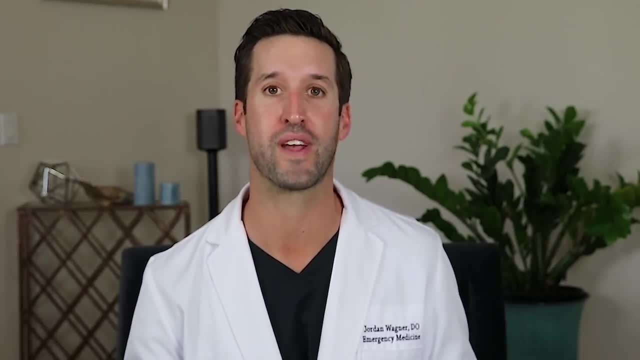 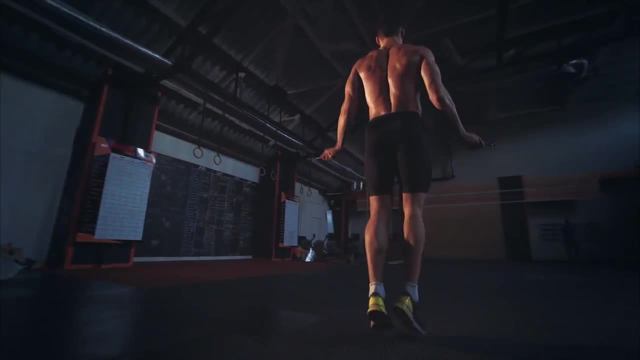 My favorite amino acid supplement that I am currently using for my workouts is a product called Perform by The Amino Company. Working overnight at the hospital, I usually find myself working out at off times. Thus I use Perform, as it gives me a type of mental 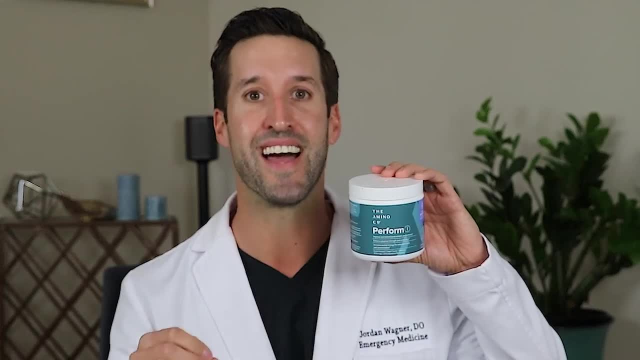 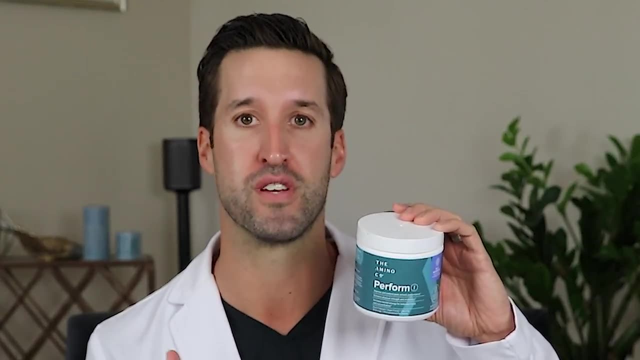 clarity and concentration that I need for my workouts. I like this formulation due to the fact that it contains the ideal ratio of neurotransmitter precursors for optimal brain function, as well as creatine and caffeine in it. It also works to reduce fatigue and dehydration. 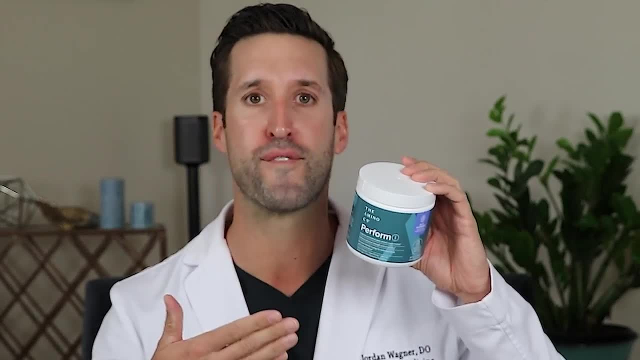 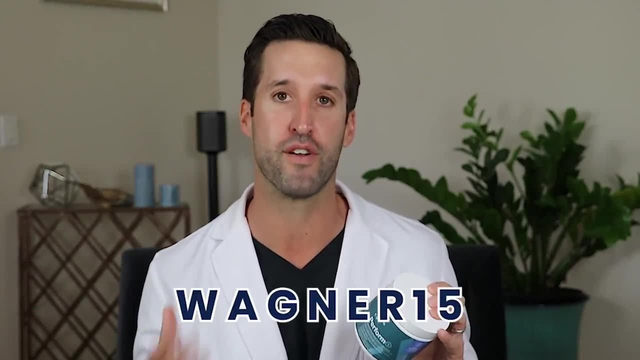 and it minimizes recovery times. It's all vegan, it's gluten-free and keto-friendly. I'll put the link in the description below for you guys to check it out. If you're interested in it, you can use the code WAGNER15 for 15% off. BCAAs or branched-chain amino acids, have been. 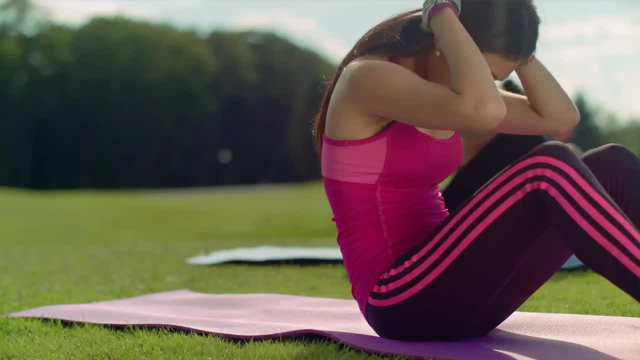 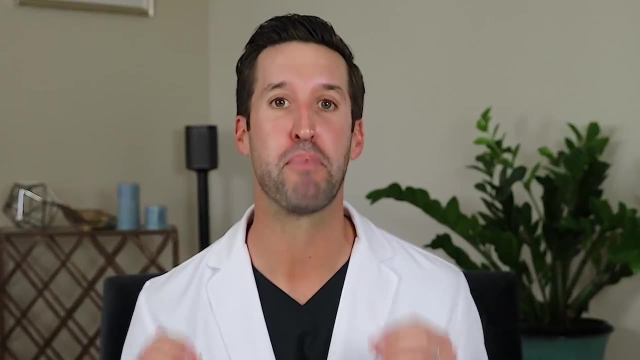 shown to decrease muscle damage. Therefore, supplementing with BCAAs, especially before exercise, may speed up recovery times. Number four: increased muscle growth. One of the most popular uses of branched-chain amino acids is to increase muscle growth. The. 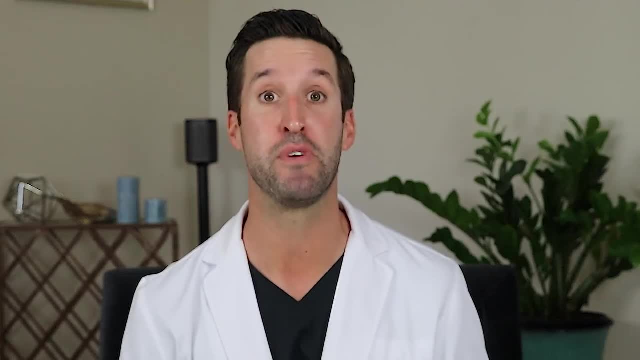 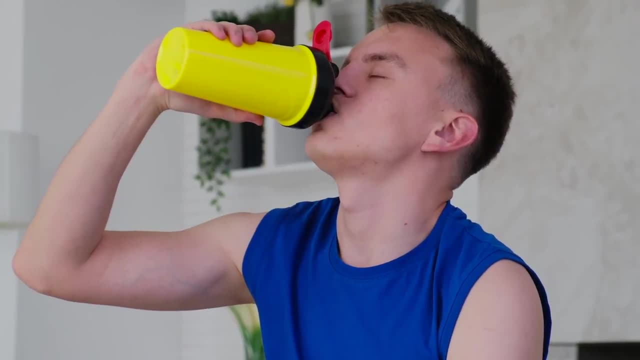 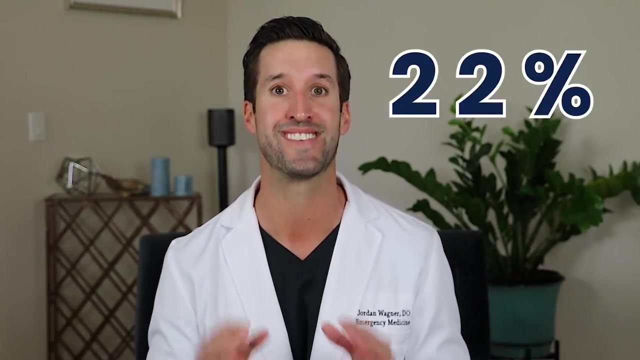 BCAA leucine activates a pathway in the body that stimulates muscle protein synthesis, which is a process of making muscles. In one study, people who consumed a drink with 5.6 grams of BCAAs after their resistance workout had a 22% greater increase in muscle protein synthesis compared to those who 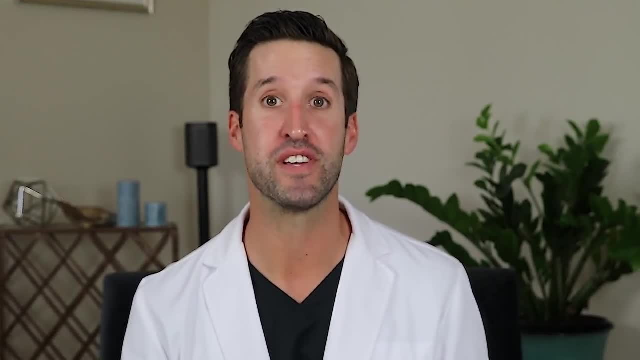 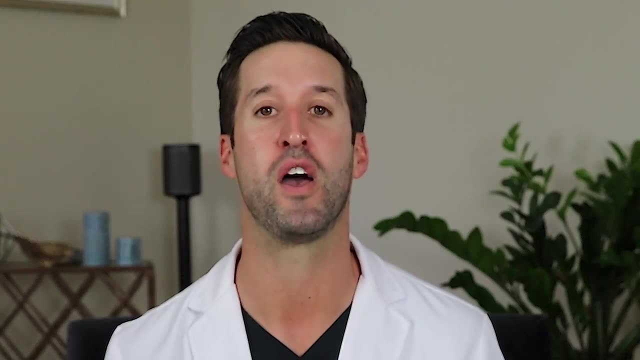 consumed a placebo drink. That being said, this increase in muscle protein synthesis is approximately 50% less than what was observed in other studies where people consumed a whey protein shake containing a similar amount of BCAAs. Number five amino acids benefit people. 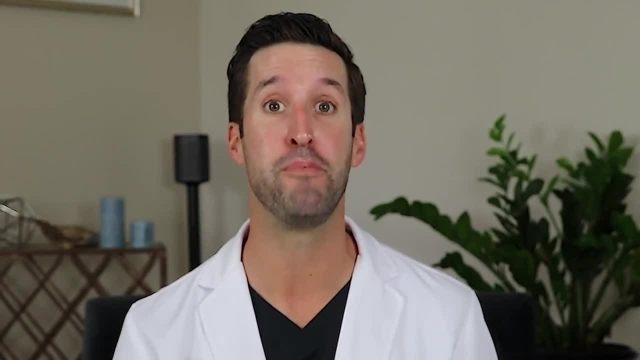 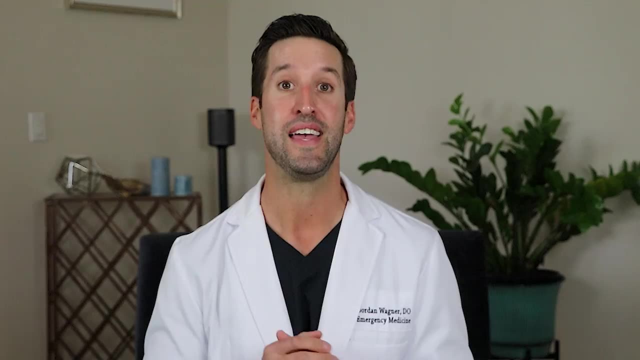 with liver disease. That's right: liver disease. Branched-chain amino acids may improve health in people with cirrhosis, a chronic disease in which the liver does not function properly. It's estimated that 50% of people with cirrhosis will develop hepatic encephalopathy. 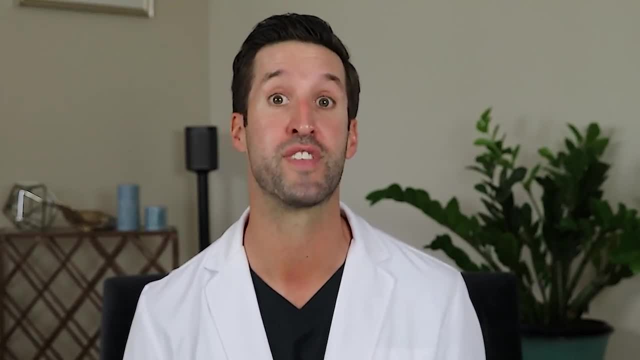 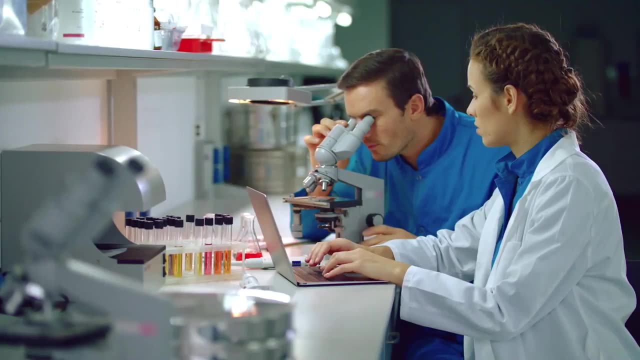 which is a loss of brain function that occurs when the liver is unable to remove toxins from the blood, While certain sugars, like lactulose, are the mainstays of treatment for hepatic encephalopathy. therefore, researchers have recommended amino acids as a nutritional 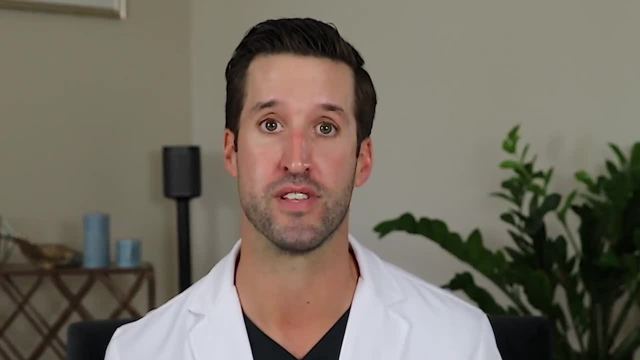 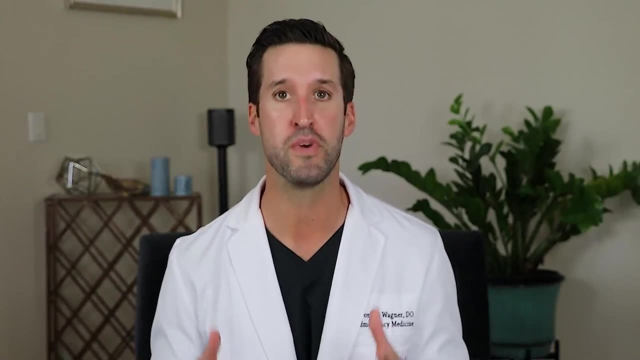 intervention for liver disease Number six: low-carb, low-carb, low-carb, low-carb, low-carb liver disease patients to prevent complications. All right, I know I just threw a ton of information out to you, but amino acids are essential. We all need it in our diet. Consuming amino acids.